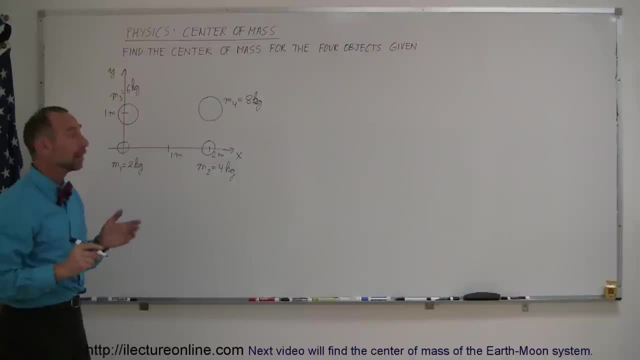 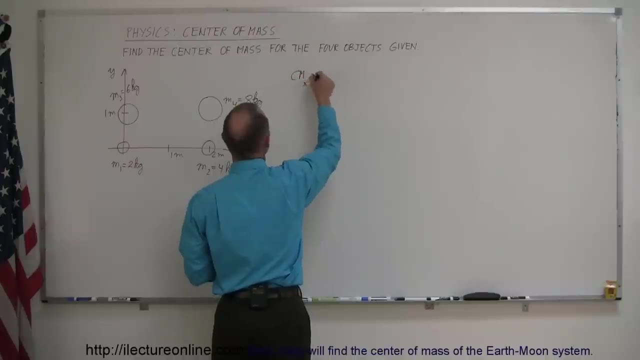 considered to be located at that exact point indicated. then the way you find the center mass- you have to do each direction separately- is as follows: The center of mass in the x direction is equal to the sum of the product of the masses of each object, so I'll say mass of i. 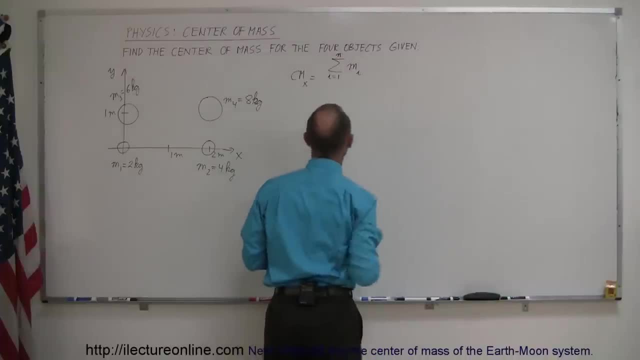 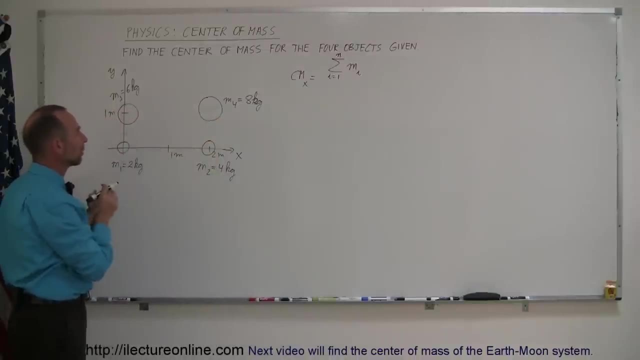 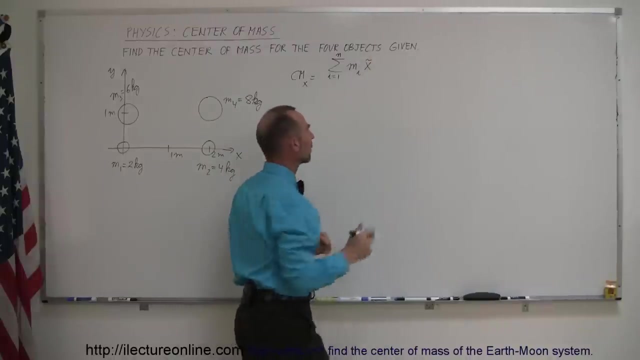 from i equals one to n, however many there are multiplied times the x coordinate of the mass of each of these items. So you could say that would be x, and I like to put a little like squiggly line on it something I learned a long time ago from a teacher. way back. 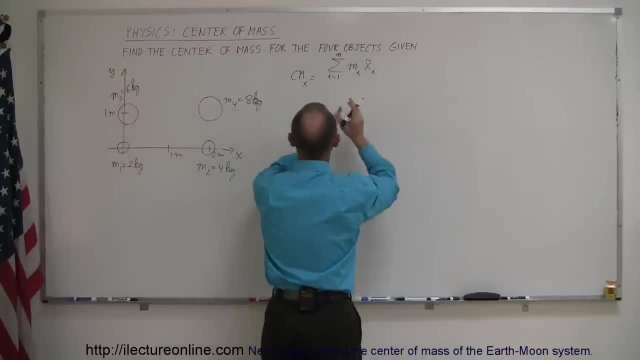 and so you multiply the mass of each object times the x coordinate of the center mass of each of those objects. divided by the sum of all the masses of all the objects, i equals one to n, n being of course the number of the masses that you have. 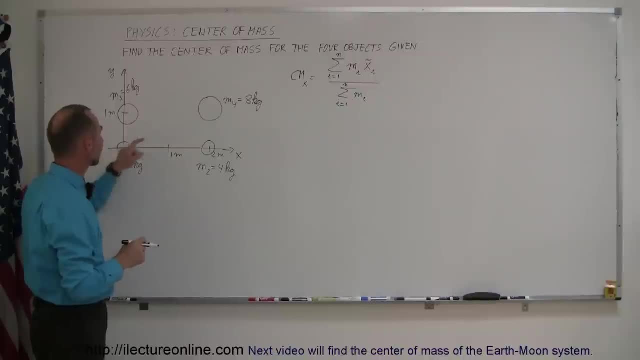 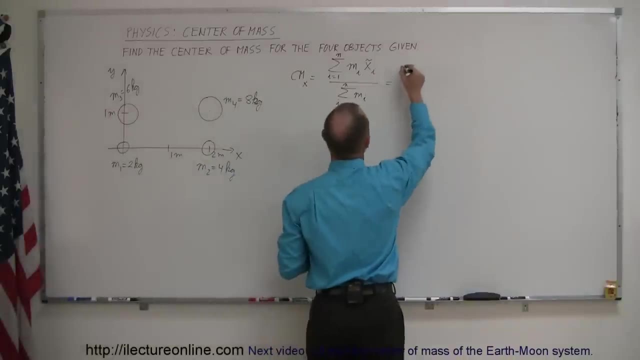 So what we're going to do in the numerator is we're going to multiply the mass of each of these times the x coordinate of the center mass of each of those. All right, let's do that. so this is equal to mass one times the x coordinate of mass one. and I might as well write: 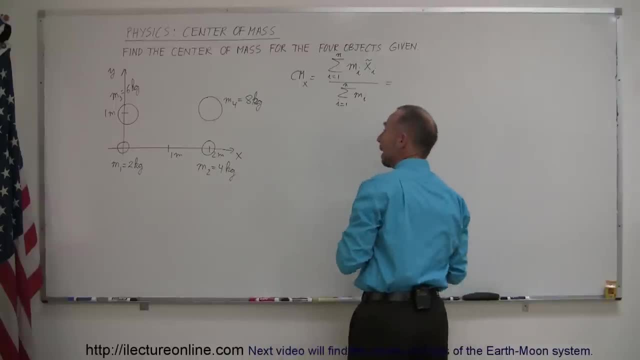 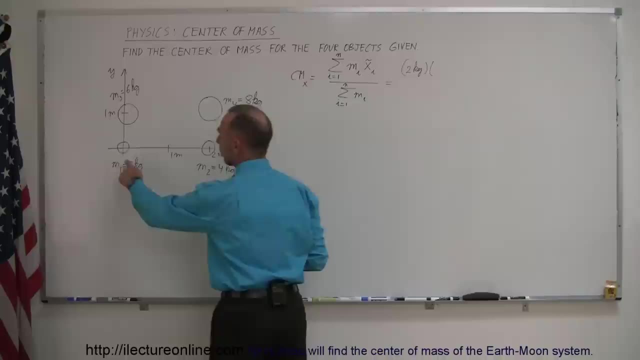 it out. let me just go ahead and do it like this. So mass one is two kilograms. I'll take two kilograms, that's mass one times the x coordinate of the center mass, and so that would be zero in this case, Plus mass two, which is this one right there, which is four kilograms. 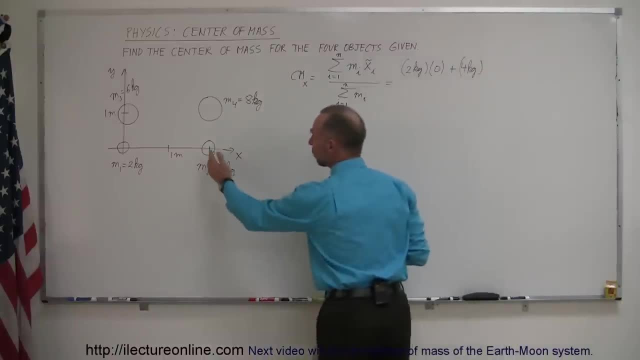 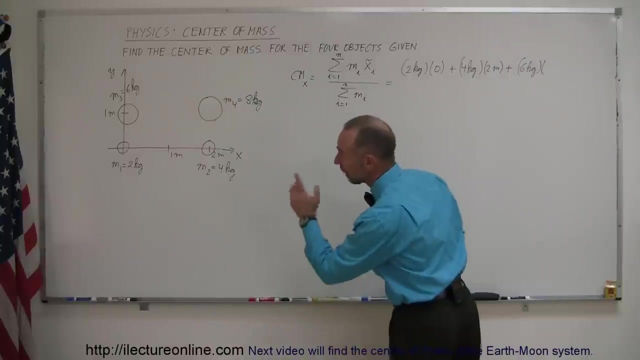 and I multiply that times the x coordinate of the center mass, and that would be two meters away from the origin. so it would be times two meters, plus the third mass, which is a six kilogram mass, and that is then also multiplied by the x coordinate center mass, which is right above. 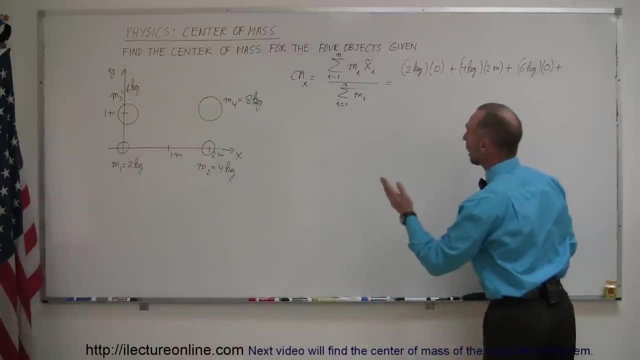 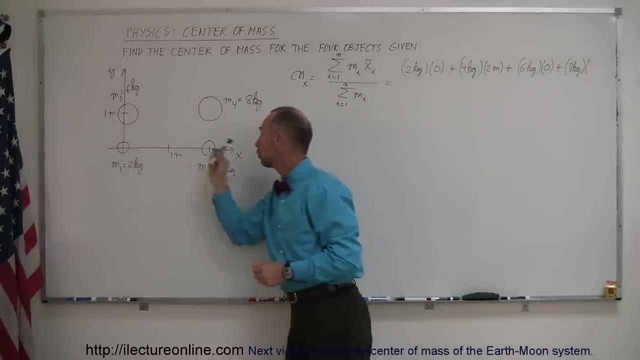 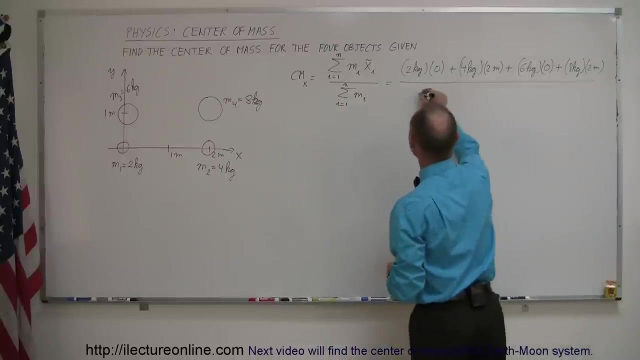 the origin, so that would be zero again, and plus the final mass, which is m4,, eight kilograms times the x coordinate of center mass, which is also two meters away. so that would be times two meters. and then we have to divide that by the sum of all the masses, so it would be the two kilograms. 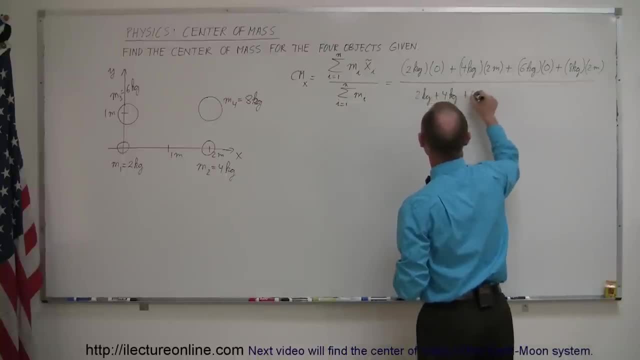 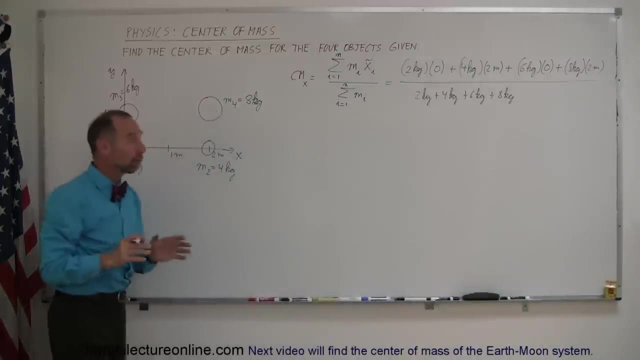 plus the four kilograms, plus the six kilograms, plus the eight kilograms. All right, so quickly recap of what we did. we had four masses, each had its individual mass, that were located at four different positions. each mass was one kilogram. 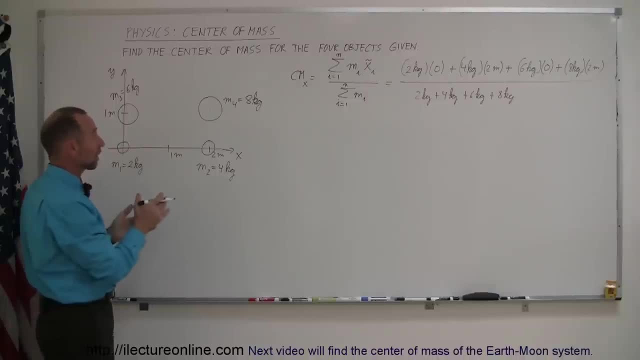 of course has an x and y coordinate, and to find the center mass in the x direction we have to multiply the mass of each of the masses times the x coordinate of each of their center masses and then divide that by the sum of all the masses. so let's go ahead and do that, so this is equal to: 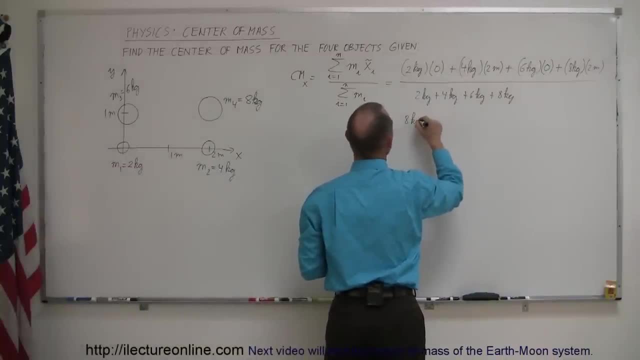 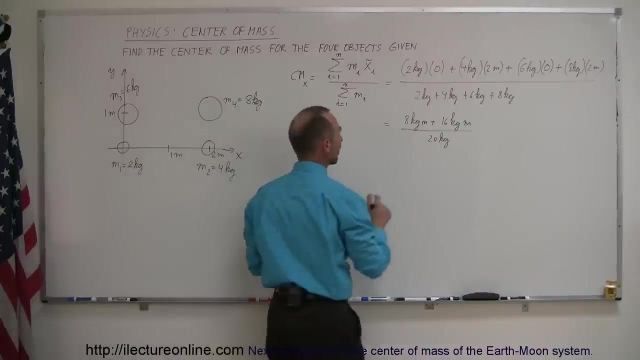 that's zero, that's eight kilogram meters. plus that would be 16 kilogram meters. divided by that's 10, that's 20 kilograms. and notice that the kilograms cancel out and we're left with 24 divided by 20, which 24 divided by 20, which would be 1.2, 1.2 meters. so the center mass in the x 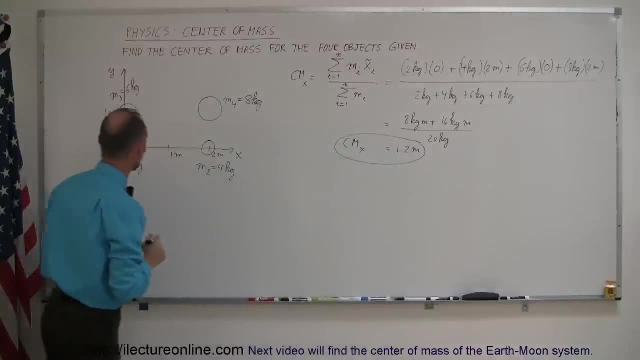 direction is 1.2 meters to the right of the origin, so this is one meter. this is 1.2 meters, so be right around here somewhere. so the center mass would be somewhere along this line. we just don't know how high it is in the y direction. that will, of course, depend upon. finding the center mass in the y direction. so doing everything again. now for the y direction, the center mass. the y coordinate of the center mass is equal to the sum from: i equals 1 to n of all the masses times the y coordinate of the center masses of each of those, and divide that: 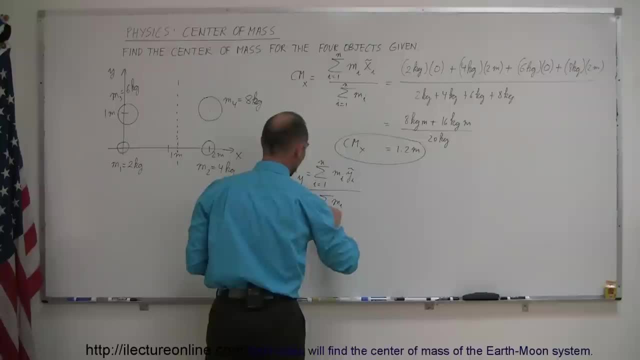 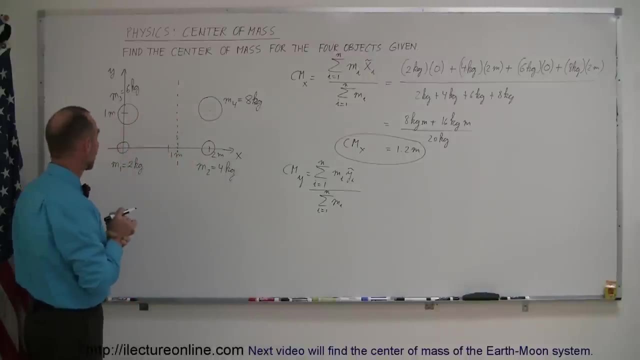 all by the sum of all the masses from i equals 1 to n. again, we're going to multiply each mass times the y coordinate of the center mass of each. okay, so doing that again, starting with mass one, that's equal to two kilograms times the y. 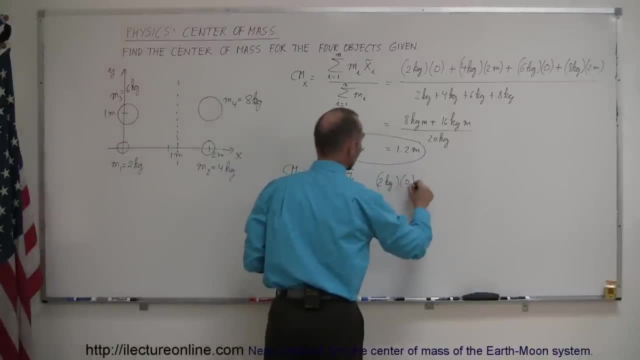 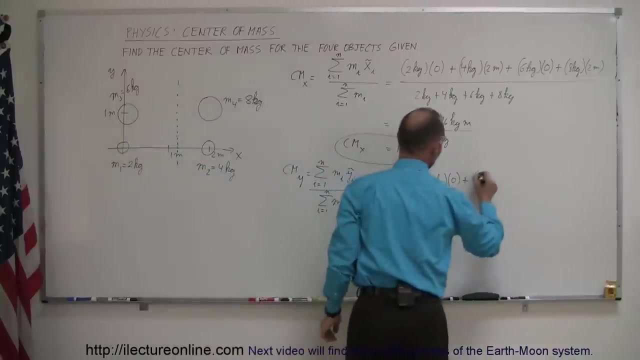 coordinate center mass, and since that's the origin, that will be zero as well, plus the second mass, which is four kilograms, and that's then multiplied times the y coordinate center mass. but since it's on the x-axis, that is also zero, plus the third mass, which is right here, six kilograms. now that 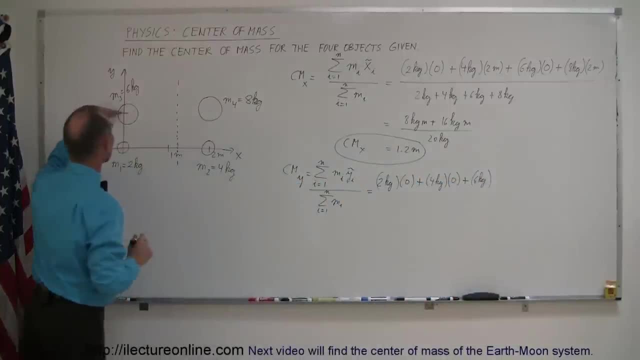 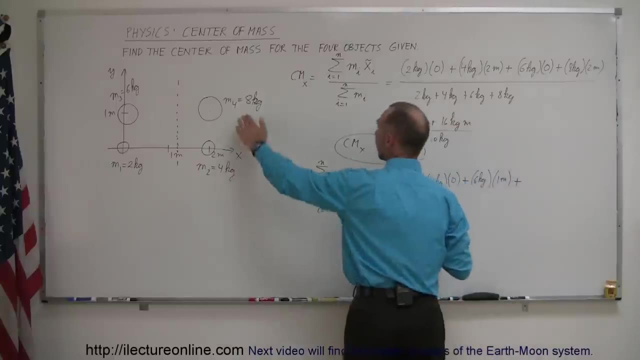 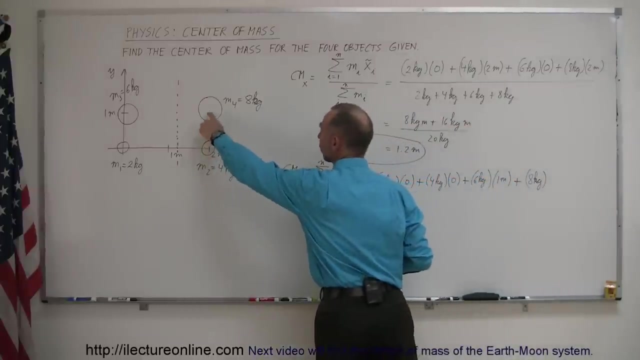 one is above the x-axis, so it's one meter above the axis. so the center mass in the y direction is one meter, plus the final mass which is eight kilograms, and it also is one meter above the x-axis. so the center mass of this mass in the y direction is also one meter and we divide the.